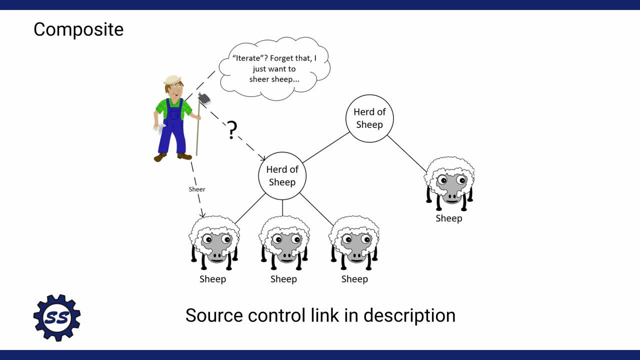 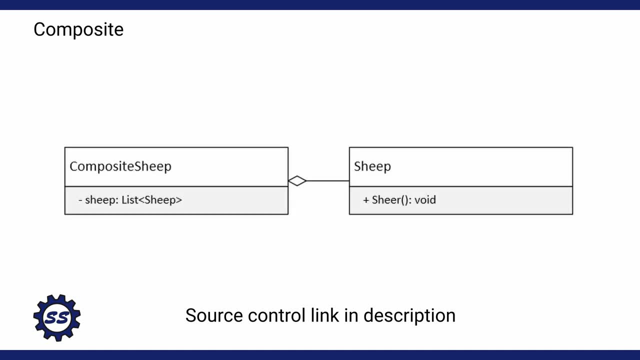 that group that are in the group. So that's a lot of work for the farmer And all the farmer wants to do is shear the sheep. So instead, what we can do is introduce a composite object, So in this case a composite sheep object that contains sheep inside of it in something like a list. 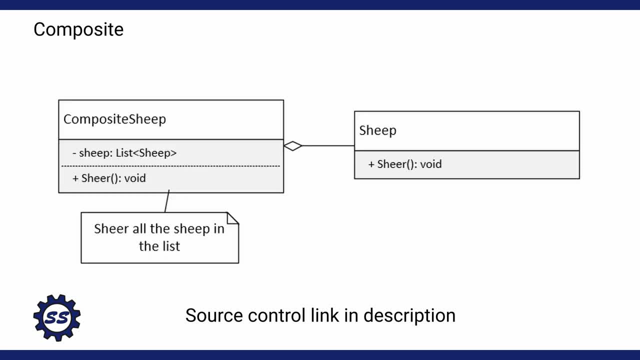 And then that composite sheep can have a shear method And that shear method will shear all of the sub sheep. So that's kind of a silly example. But the main benefit here is that the farmer can receive some kind of sheep or a composite sheep And since that composite 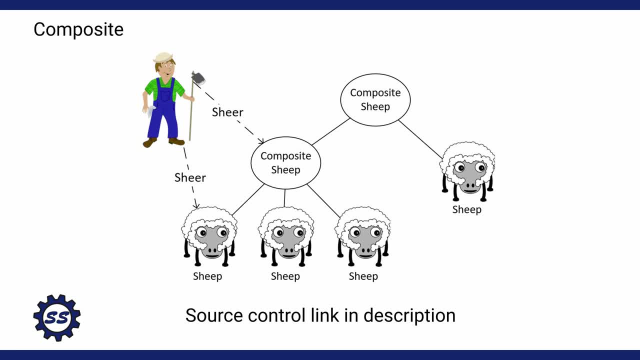 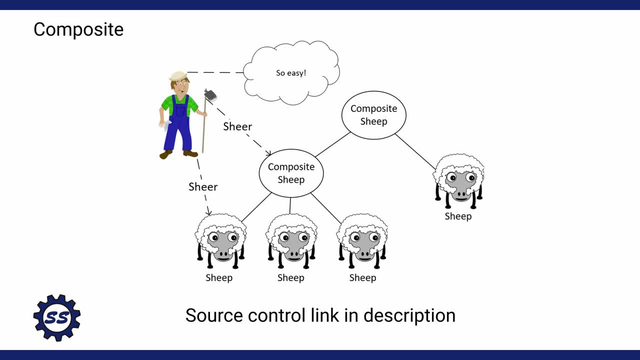 sheep has a shear method on it. it's not going to have to iterate over all the sub sheep, And the farmer won't even have to care if it's dealing with an individual sheep or a group of sheep. All it's got to do is call shear and all the sheep will be sheared. So let's implement this. with what? 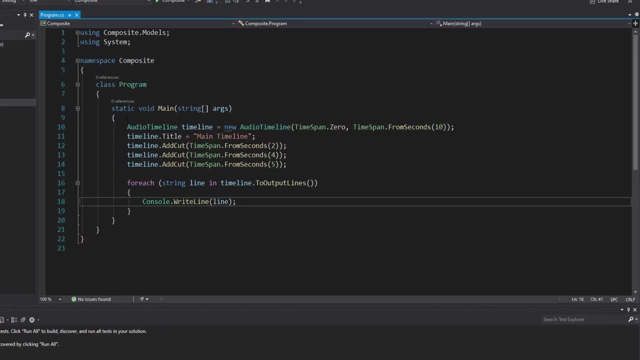 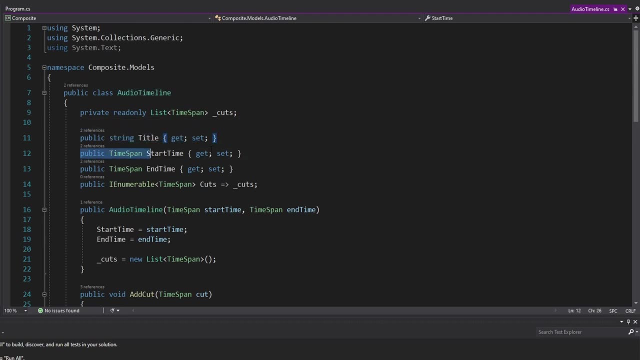 is hopefully a better example. So I have an audio timeline and this is actually inspired on a project I've been working on. Let's actually look at our audio timeline So it can have a title, a start time, an end time and 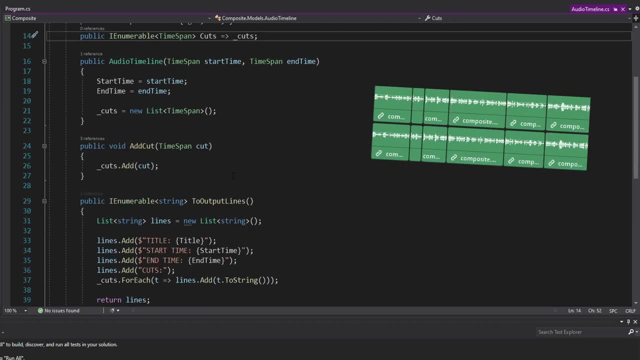 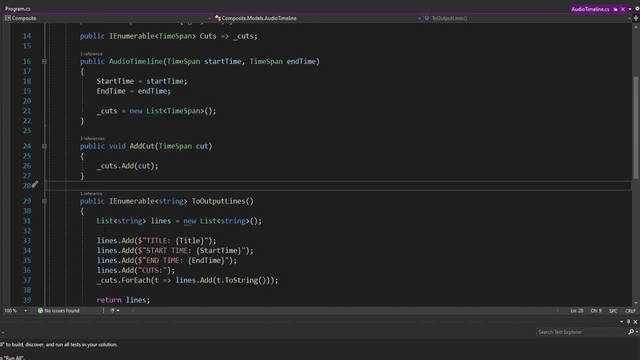 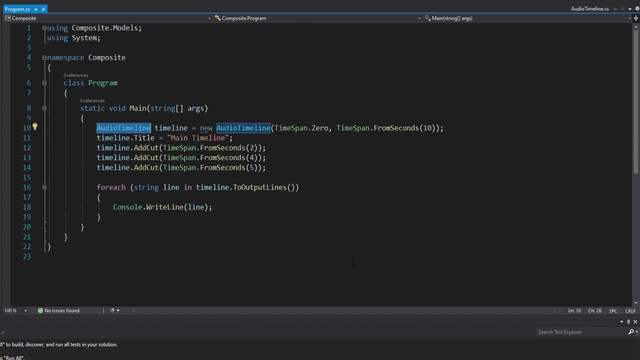 it's made up of a bunch of cuts And of course, we can add a cut And then we have a method to output lines, And this will give us a list of strings that represent the data or information about this audio timeline, And I want to use this information to maybe write it to a file so that I could import. 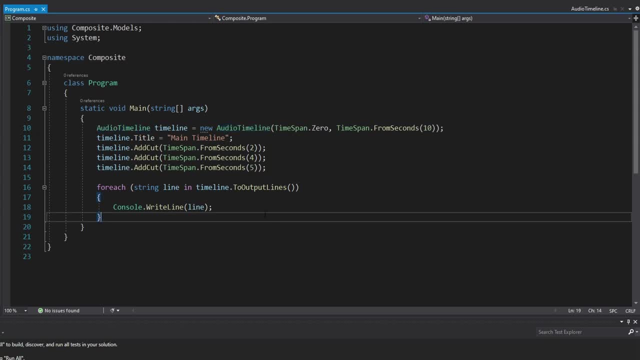 it into my video editing software, But we're not going to be doing that here, We're just going to write it to the console. Anyways, I have this individual audio timeline, But in reality a timeline could be made up of many. 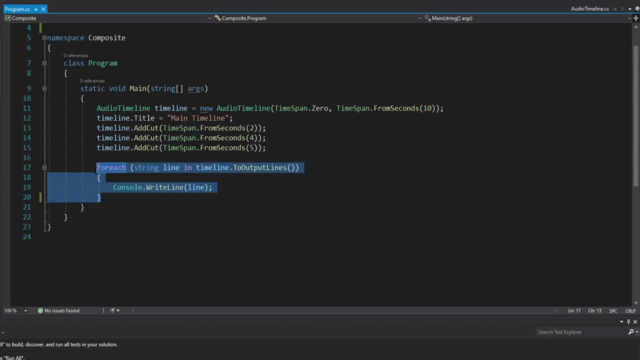 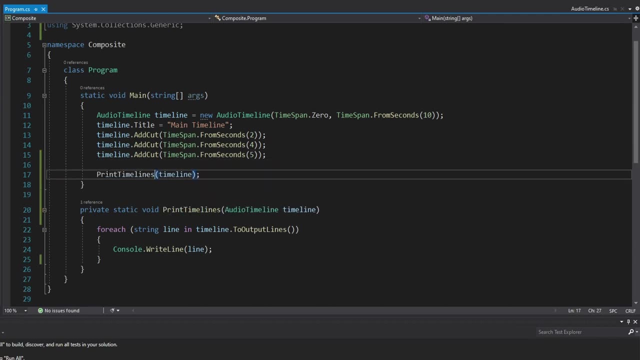 timelines. So actually, before we go a little bit further, let me extract this to a method so that we can see this pattern a little bit better and why it can be helpful here. So this will be print timeline And of course, this takes an audio timeline. Now, if I were to support the idea that 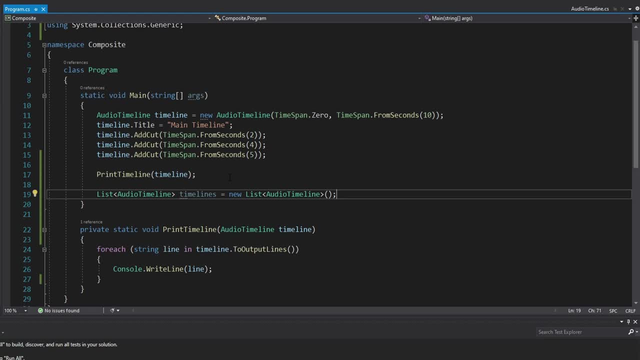 a timeline can be made up of many timelines. I might think at first, okay, I'll just have a list of audio timelines, But then if I wanted to print this composite timeline, I wouldn't be able to pass it to the print timeline. 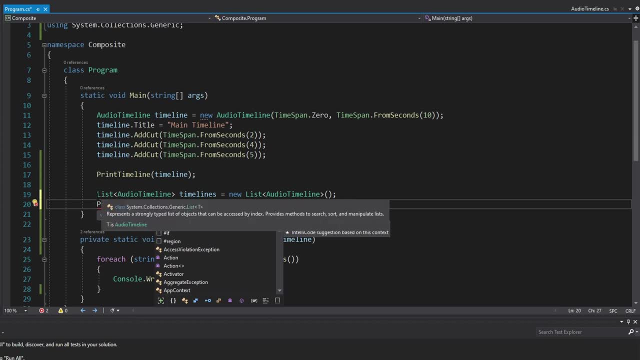 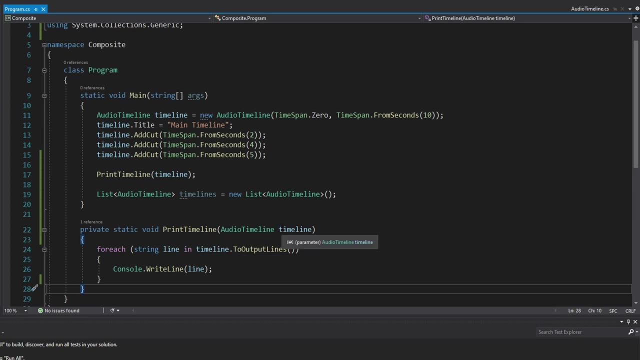 method, because this takes just an audio timeline. It doesn't take a list of audio timelines. But let's take a look at what this print timeline method needs. All it needs is a method on the timeline to output lines. So what I can do is actually extract this method into an interface like an iAudio timeline. 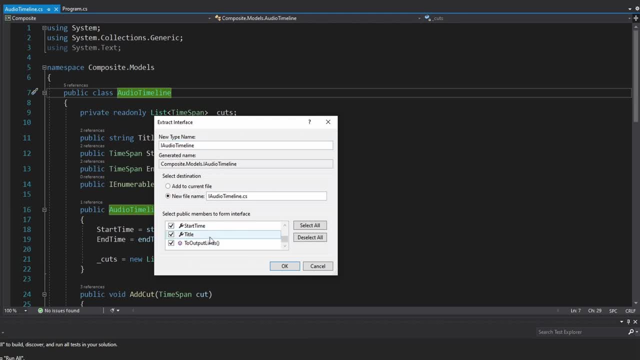 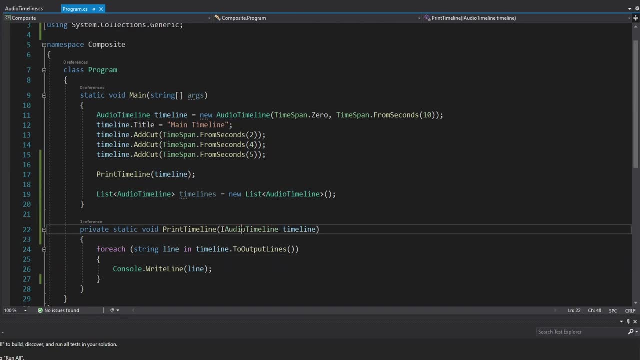 So let's go ahead and do that. So all an iAudio timeline will need is two output lines. So I'm going to use two output lines And now my method can take an iAudio timeline, And since we only need an iAudio, 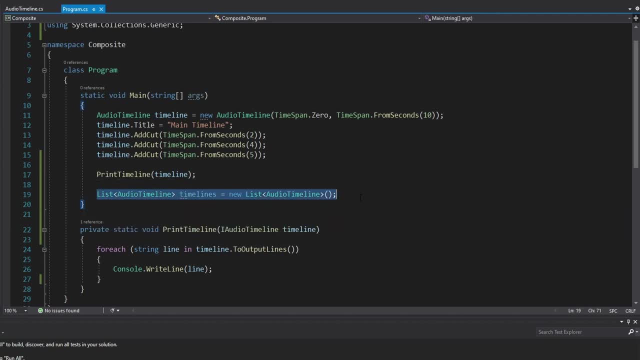 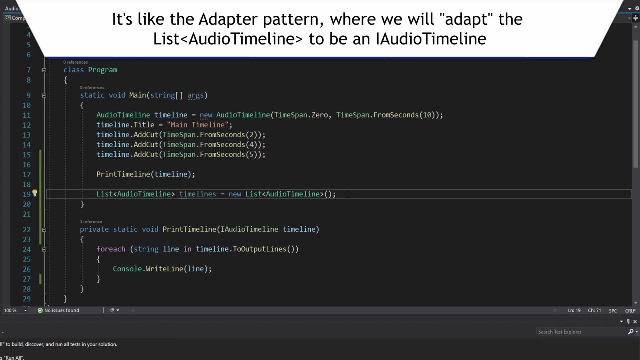 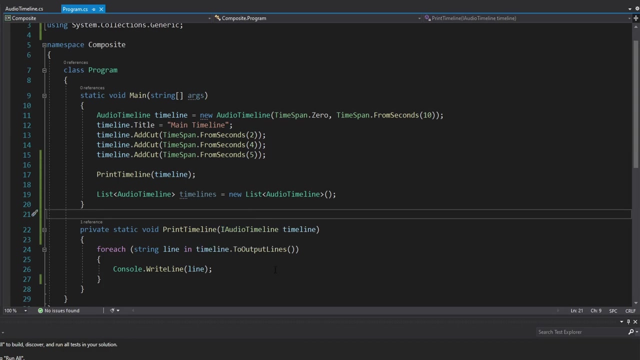 timeline. here what I can do is encapsulate this list in an object that implements the iAudio timeline interface, And that object will be our composite audio timeline, And then I'll be able to pass in my composite audio timeline to this print timeline method And it'll call the two output. 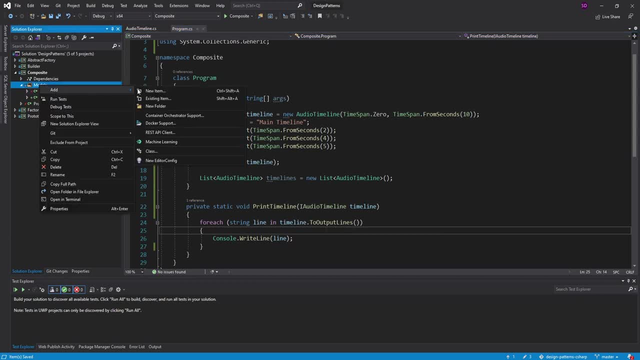 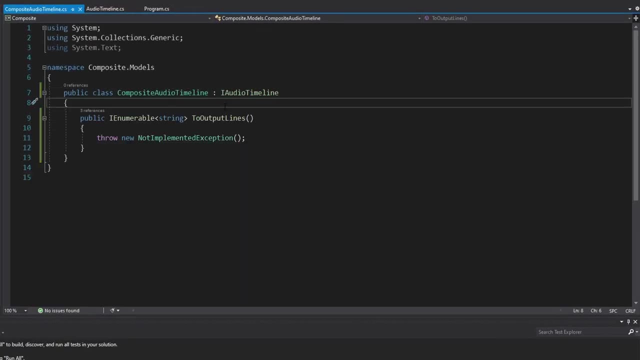 lines method that we implement on our composite. So let's create our composite audio timeline, just a class for that, implementing the iAudioTimeline interface. And of course, this object will encapsulate our list of audio timelines. So let's move those into the class as a field. 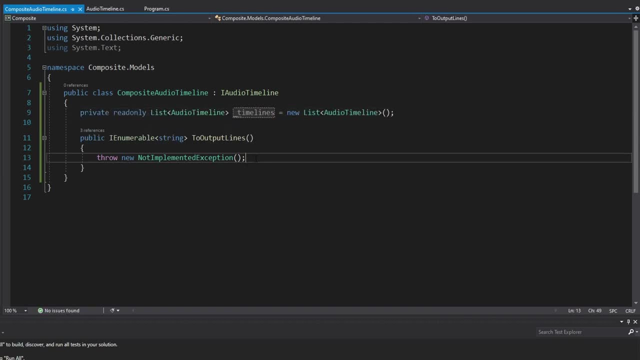 We can even make it read-only, But of course, we still need to implement this toOutputLines method. And how would we output a composite audio timeline? Well, in this case, all we're going to do is iterate over all the timelines in our composite object. 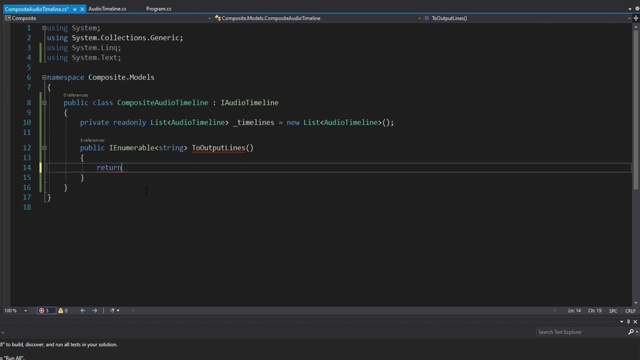 Actually, I'm just going to do some good old-fashioned link here, So we'll take our timelines that are inside this composite and map those with select to each timeline's toOutputLines method. Actually, this is not correct. This gives us back an iEnumerable of an iEnumerable of string. 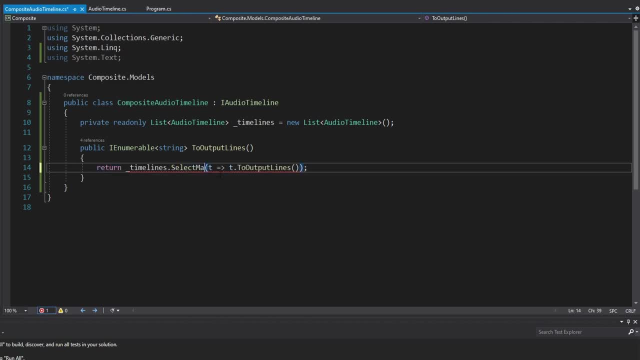 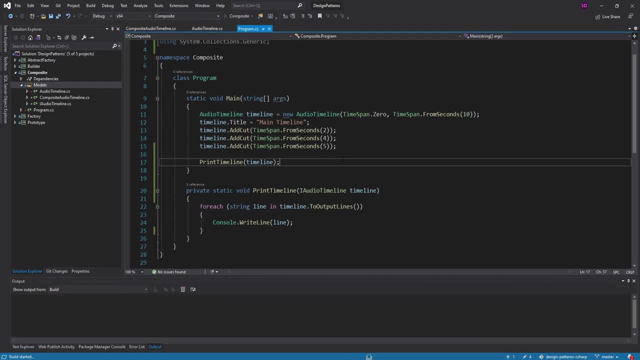 So that's the output of each timeline. So actually we have to do selectMany so that we join all of that output together. So let's begin using our composite. And actually, before I remove this, let me actually show off what's going on here. 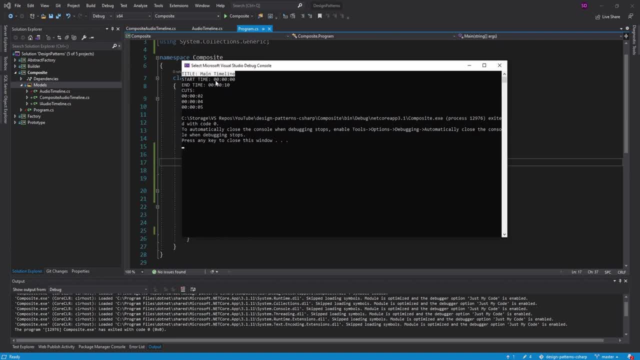 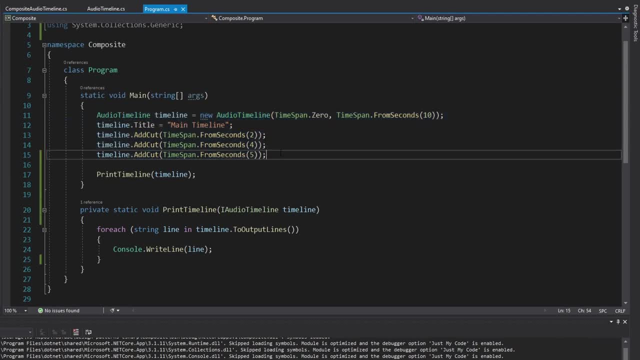 So printing a timeline just shows the timeline, The timeline's title, the start time and end time and then all the cuts that we've added to the timeline. So let's actually get a few timelines in here And then we will create a composite timeline. 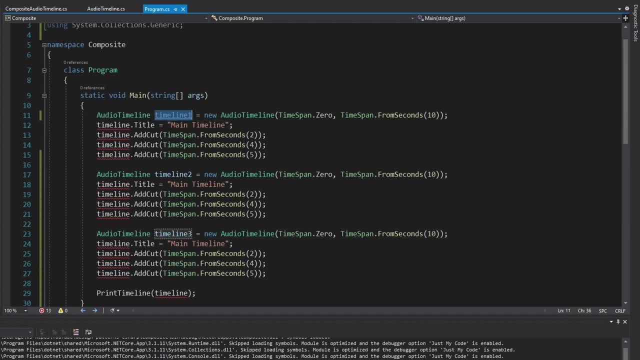 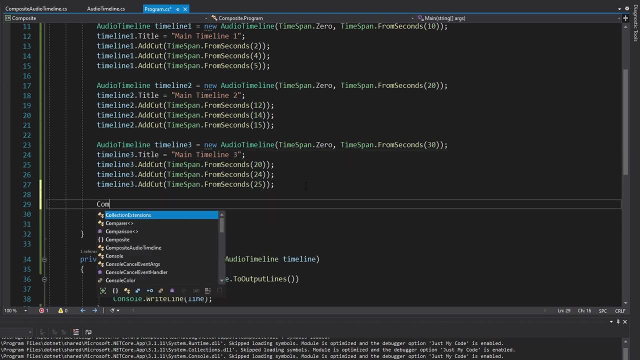 So I'll call these timeline 1,, 2, and 3.. Update these names And we'll add some variation to all these. And there we go. So let's turn these into a composite timeline. So I'll get a composite audio timeline. 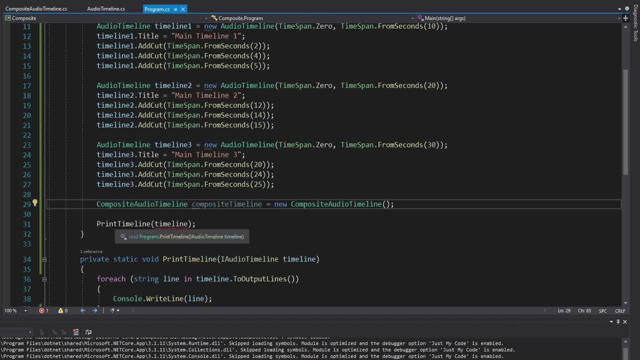 Just instantiate that And then my print timeline I'll pass in my composite timeline And since this implements the iAudioTimeline interface, we can indeed pass it to the method. But first I need to add all of these individual timelines to my composite timeline. 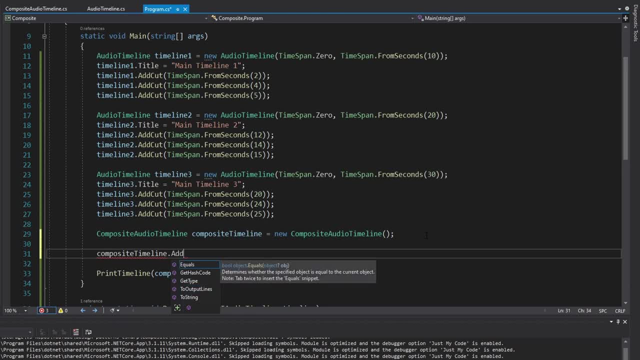 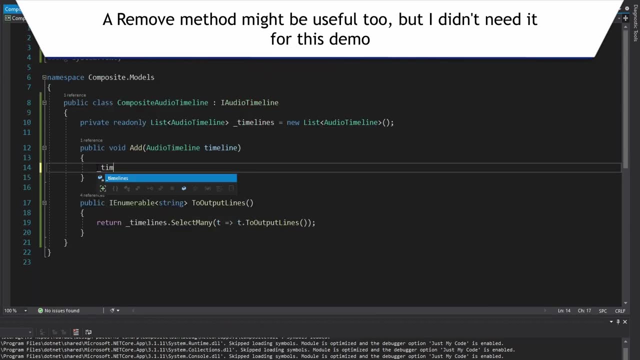 So the best way to do that, we will just generate an add method on our composite audio timeline So we can generate that And all we have to do in here is add the timeline that gets passed to this add method to our timeline's list. 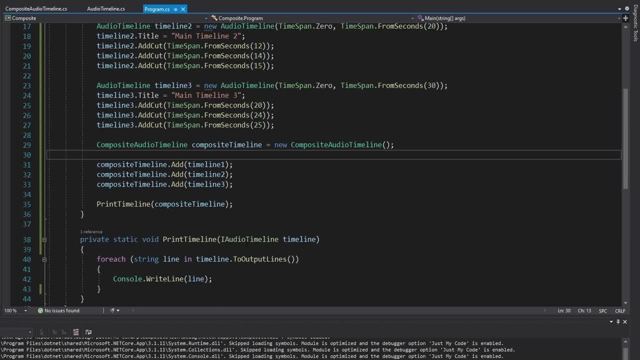 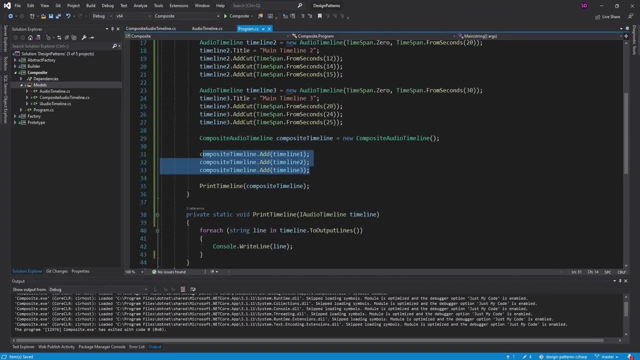 And let's add the rest of our timeline. Okay, so the audio timeline that we pass in, which is the composite, should give us back all of the output lines for all of the sub-timelines within the composite. And there we go. 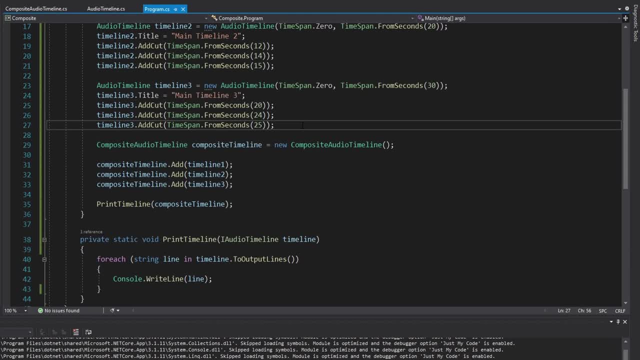 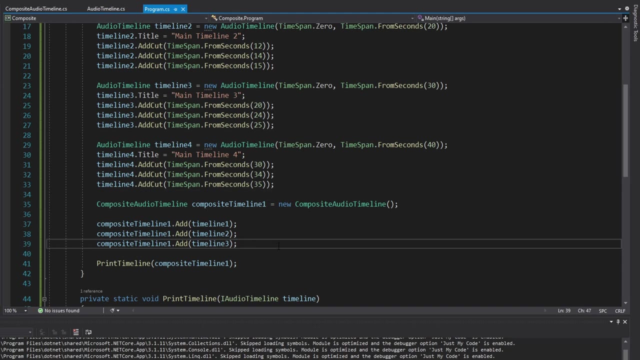 We do print all of the timelines, Alright. so we kind of got what we want. But another thing to consider is that a composite audio timeline should also be able to be made up of other composite audio timelines. Alright, so for my first composite timeline, what I'm going to do is remove timeline 3.. 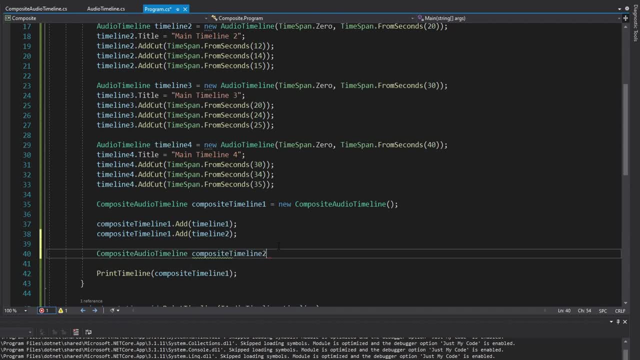 And then we're going to create another composite audio timeline, composite timeline 2.. And for this composite we're going to pass in timelines 3 and 4.. But I'd also like this timeline to be made up of my first composite timeline. 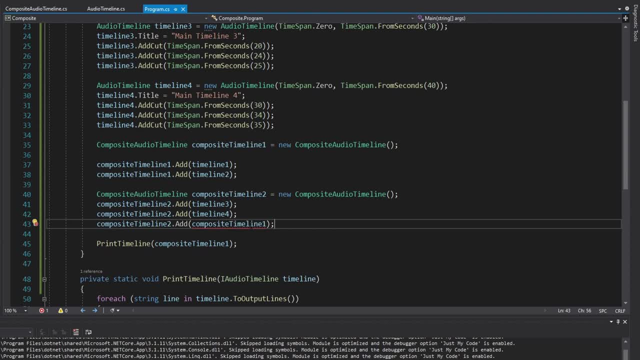 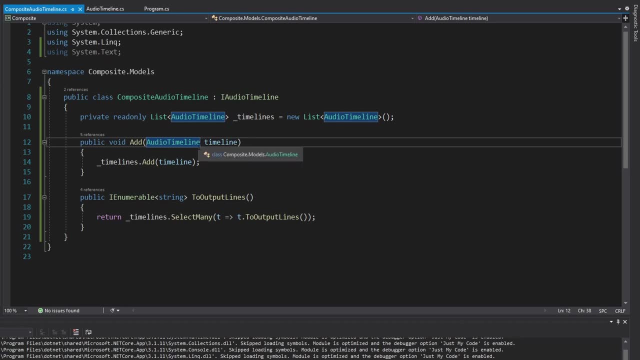 So I want to pass that in. And of course we can't pass that in Because this add method requires just a regular individual audio timeline. But we're trying to pass in a composite audio timeline But, as we recall, the composite audio timeline. 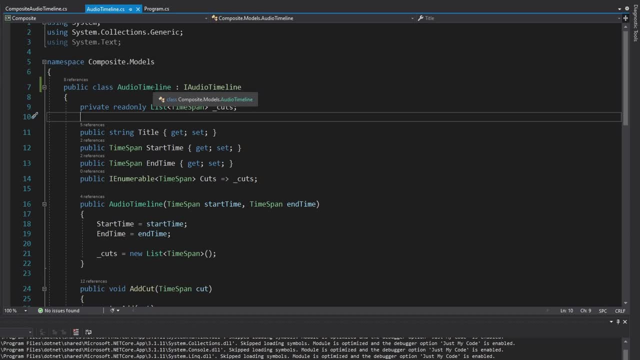 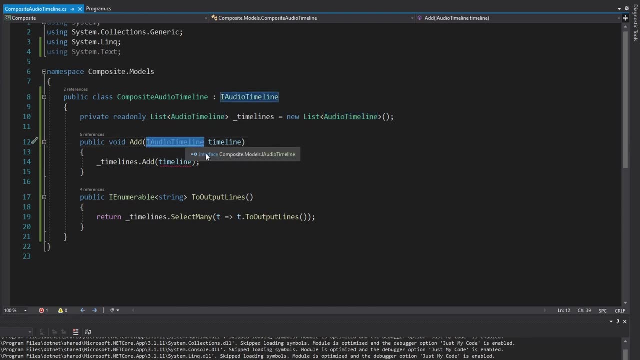 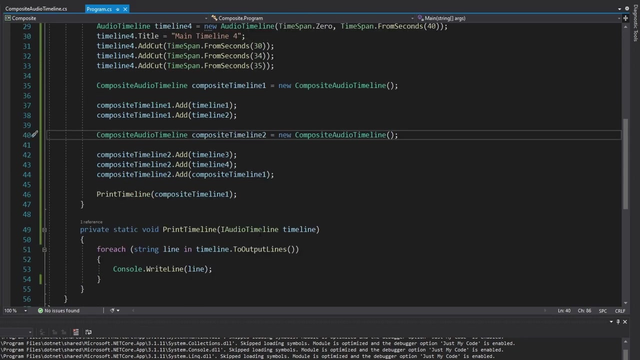 is the same as the composite audio timeline's iAudio timeline, and so does our regular individual audio timeline. So what we can do is just depend on that iAudio timeline interface, update our list to take that interface as well, And now we can pass that composite into our add method and we'll be able to print it as well. 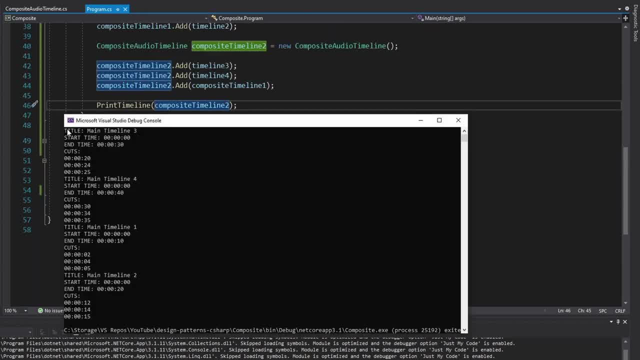 So, for print timeline, we're now going to pass in composite timeline 2.. Alright, so we printed timelines 3 and 4, because we added those to the composite timeline first, And then we're going to pass in composite timeline 1, which is made up of timeline 1 and 2.. 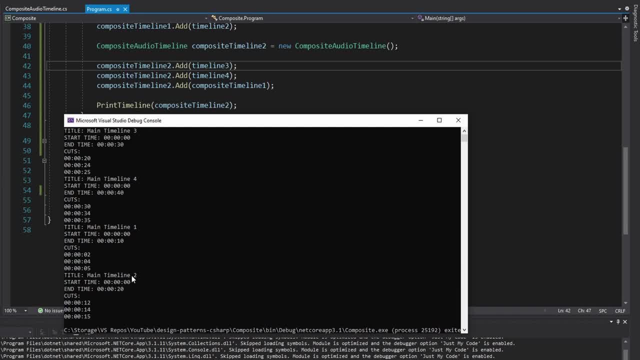 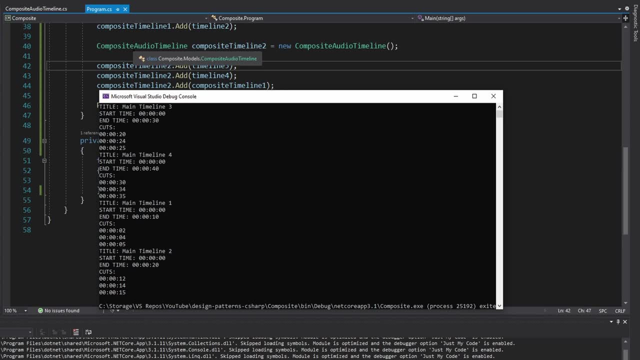 So now our composite can have composites, But I want to take this to the next level because this really isn't a pretty display of our timeline, Because this composite audio timeline it's still a timeline. So for my use case, I want all of my timelines to only have one title: one start time, one end time and then a bunch of cuts. 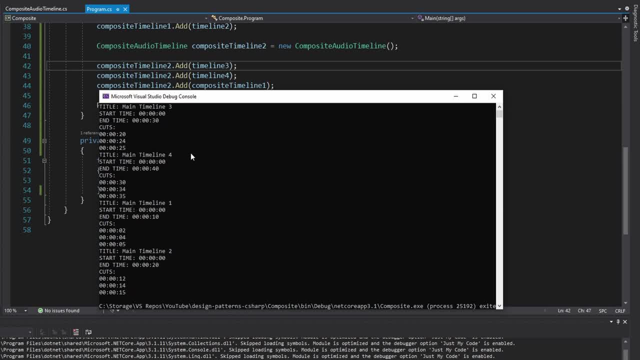 But with this display we have four titles For one audio timeline. even though it's a composite, I still only want one title, And we have four start times, four end times, So I really want to merge all of these timelines together in my composite. 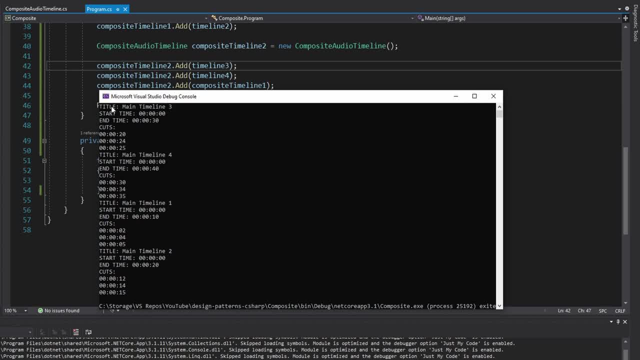 So by merging them together, we'll have one single title. The start time will be the lowest start time of all of my sub timelines, The end time will be the latest end time of all of my timelines, And then, for my cuts, I'll just have all of the cuts from all the timelines merged into one single list. 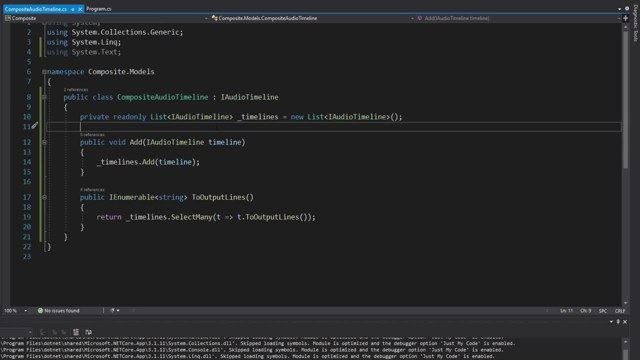 So that means my composite is going to have to be a little bit more advanced, Which is a good thing, because that shows the benefit of using the composite design pattern so that we can do complex stuff inside this class and our client doesn't have to do that. 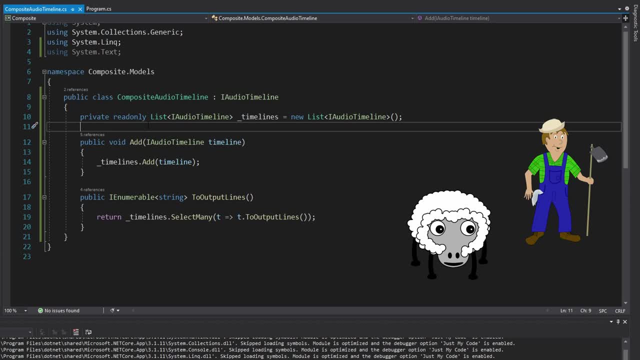 We don't want our farmer with the sheep to have to do all of the complex stuff. So we're going to have to improve this two output lines method. We're no longer just going to join all the output lines of our sub timelines, because it's just not a good representation of what our timeline is. 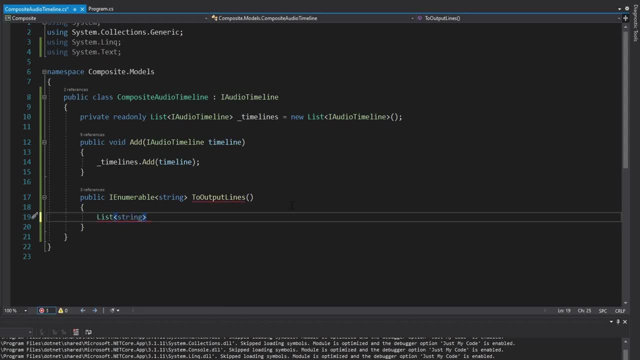 So let's just start off with a list Of what we're eventually going to return as our output, And we'll incrementally add our timeline data to this list of lines, And then, when we're done, we'll return the list of lines. 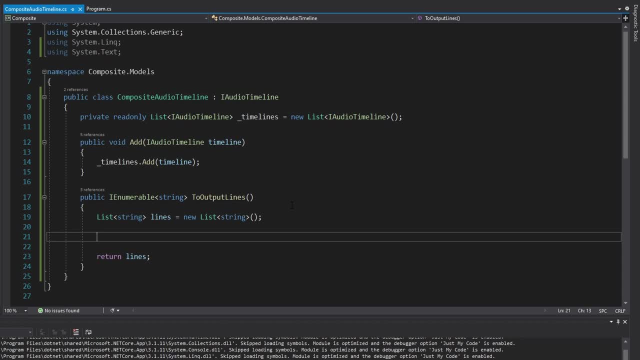 So in between here we need to do all of our work. So first, on the very first line, we want the timeline's title. So as we saw in the example, our sub timelines, they all had titles, So we could just choose one of those timelines and use that as the title. 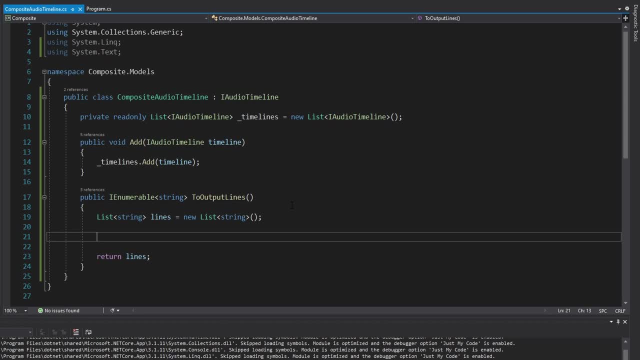 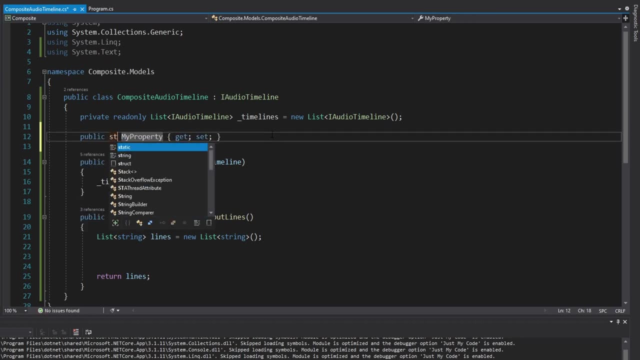 But I really don't know a good way to choose which one to use as the title. So instead, what I'm going to do is have our composite audio timeline have its own title property. So we're just going to ignore all the titles on our sub timelines. 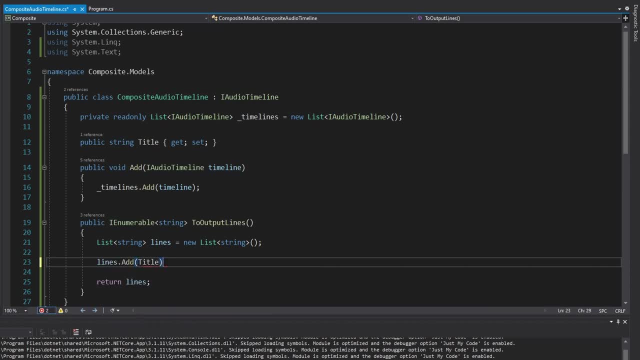 And use the title that we will eventually specify on the composite. Actually, let me do some string interpolation here, So I want this to be labeled as the title, And we're going to do string interpolation for our next few lines as well, So let's just copy that. 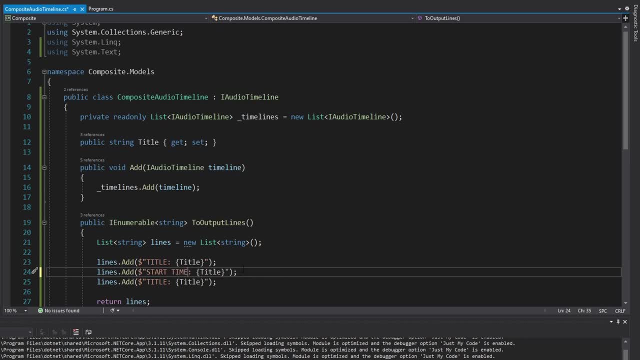 And this next line is going to be the start time of the timeline. So we had said that we want that to be the minimum start time of all of our sub timelines, So let's get those. We can use our timeline's list and use min. 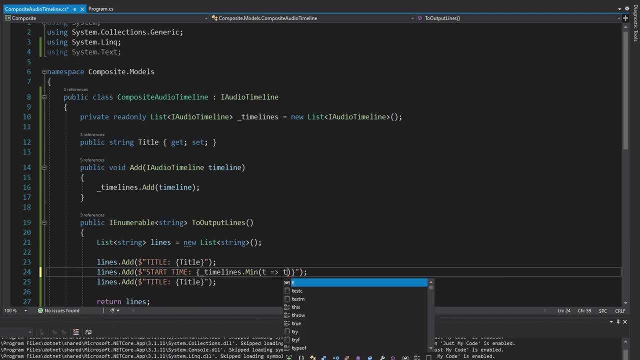 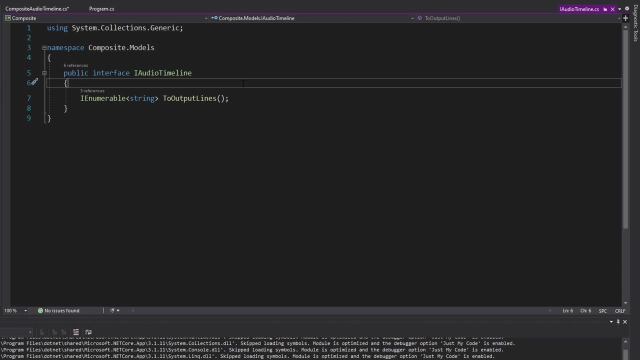 And we'll get the minimum from iterating over each timeline's start time. And uh oh, looks like our iAudio timeline doesn't have a start time member on it, So what we actually have to do is add a start time property to our iAudio timeline interface. 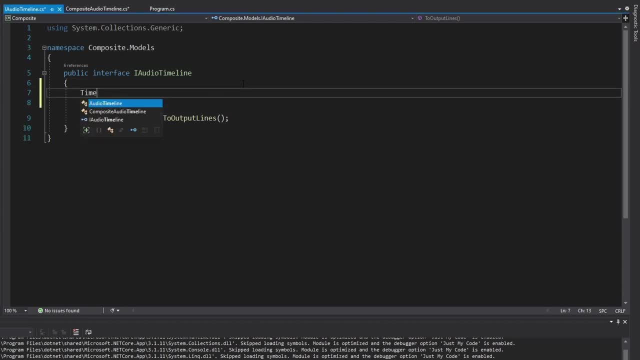 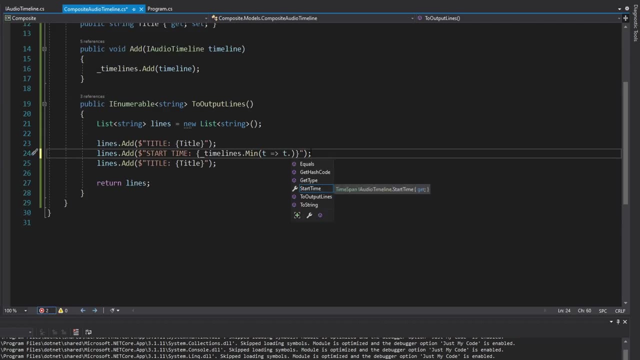 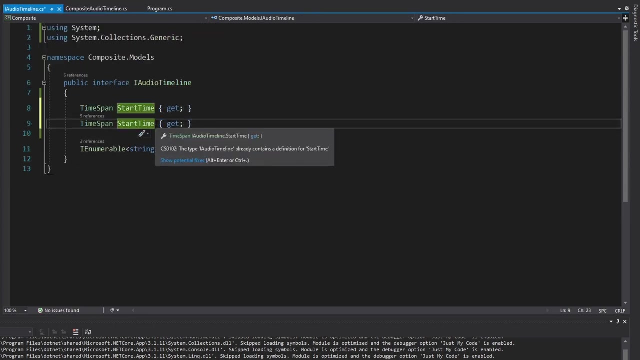 So let's just add that property. This will be a time span and a start time, And this can actually just be read- only for now, I think. So now we can access the start time property on our iAudio timelines And, while we're here, might as well add an end time as well to the iAudio timeline interface. 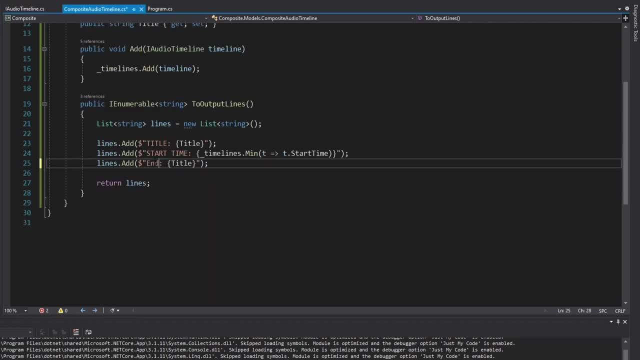 Because we're going to need that in our next line. So the end time. let me just copy this link, paste that in there. This time we're going to do max of the end time, So the latest end time. Then we're going to have to output the cuts of all of our sub timelines. 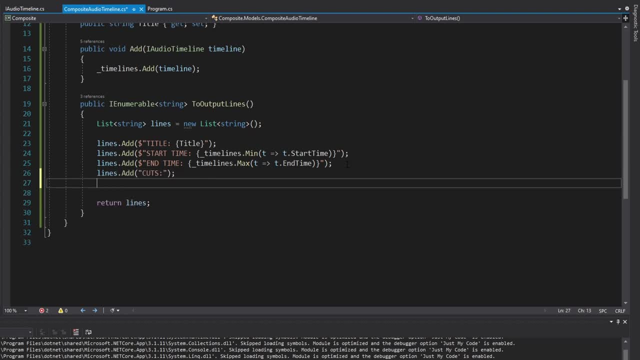 So we'll first add a header for cuts And then we'll add all the cuts from all of our timelines, So we can take our timelines, We can select all the cuts from all of the timelines, So we're going to need to select many here. 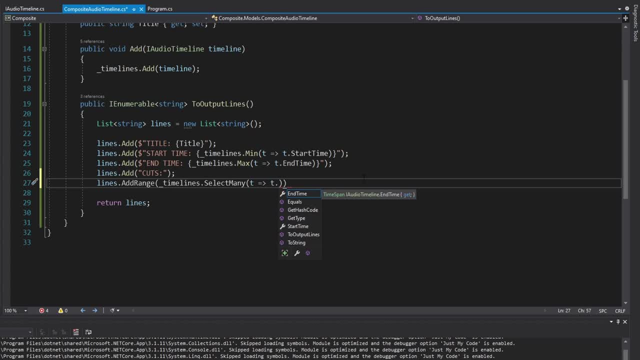 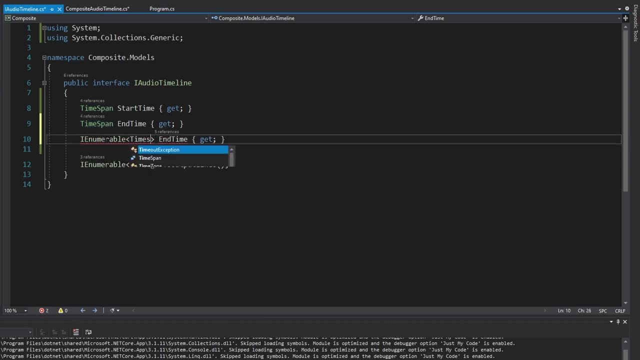 Because we are selecting many cuts And, uh oh, cuts aren't on the iAudio timeline interface either, So we're going to have to add those, Which is an iEnumerable of time spans that represent the cuts. So now we can select all those cuts. 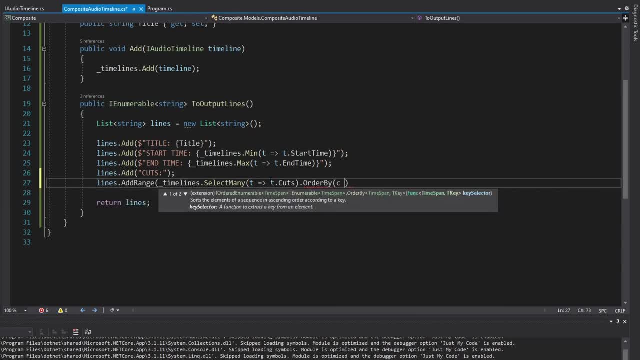 And I should also order the cuts as well. So we can do an order by, And we want to order by just the cut, And then we're adding these cuts to a list of strings, So we need to select those two strings. So we will just take each cut and call it toString. 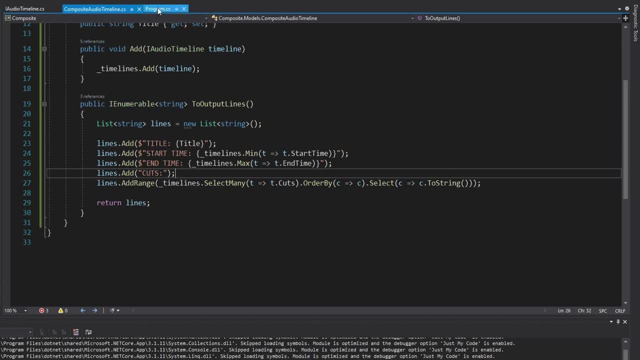 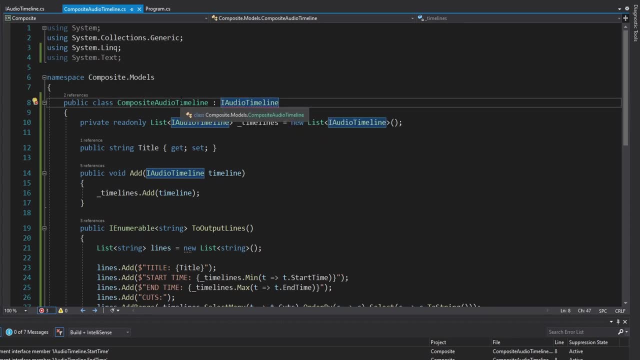 And that should be everything we need. So let's go ahead and run this. Everything should work right, And that is not correct, Because we implement the iAudio timeline interface on our composite audio timeline And we just added a bunch of required properties. 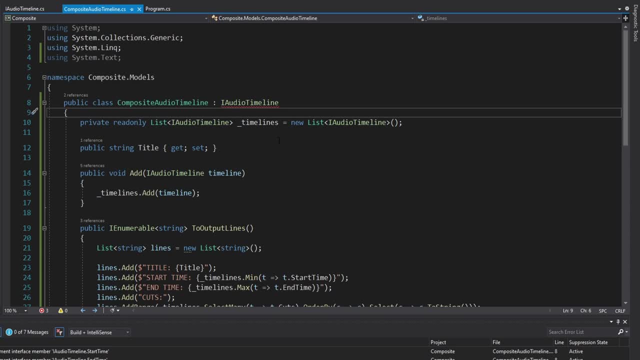 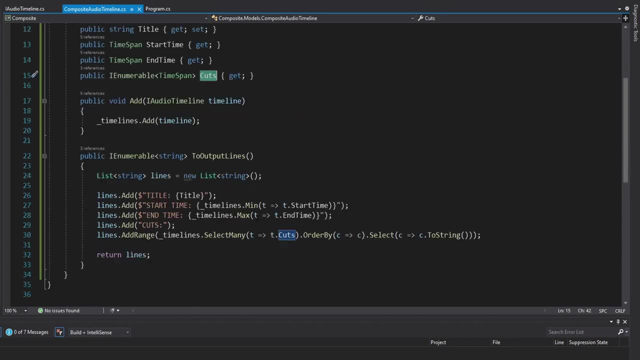 on this iAudio timeline. So we actually have to implement those properties. So let's start off by just generating them. So we need start time, end time and cuts. Well, that's no big deal because we already have those implementations kind of down here. 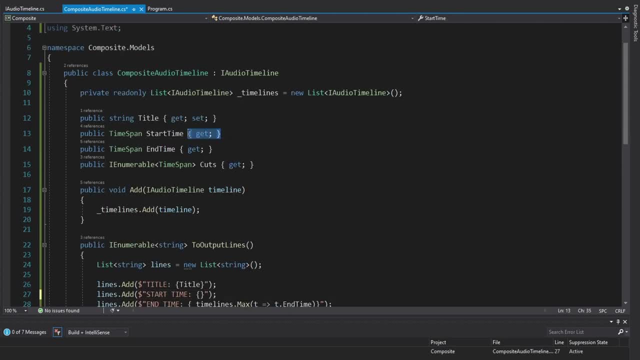 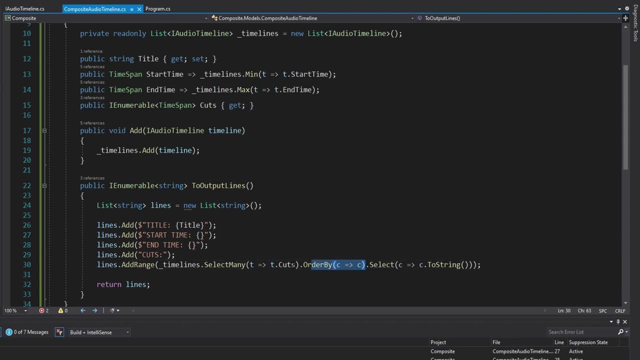 So we just cut these out. So the start time will be the minimum start time from all of the sub timelines, The end time will be the maximum end time And the cuts will just be the ordered cuts from all of the sub timelines. And now we can just use those properties down here. 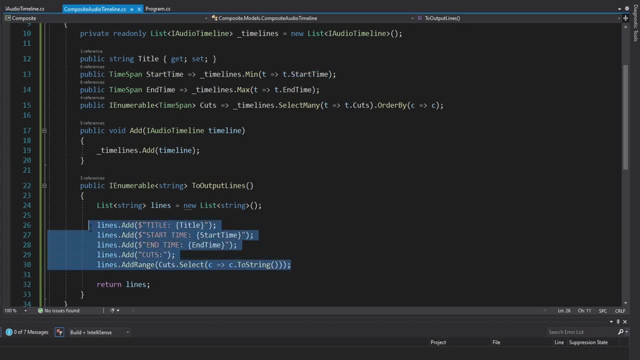 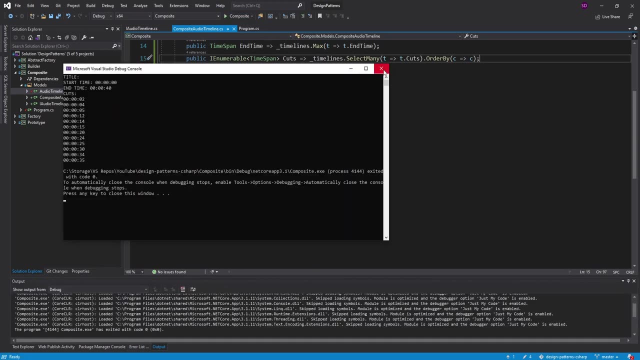 in our toOutputLines method, So this actually makes the method look a lot cleaner because we have everything in the properties. So I like that And let's see our timeline. There we go. So okay, we forgot a title. Let me add a title. 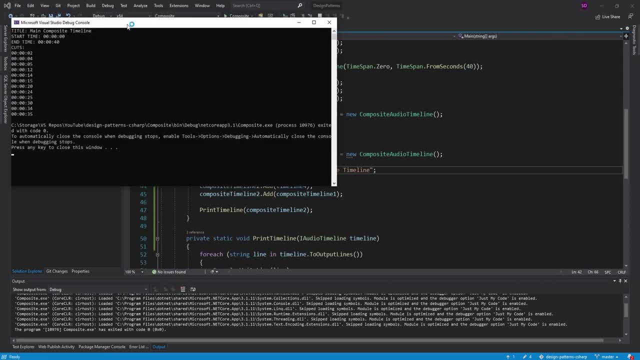 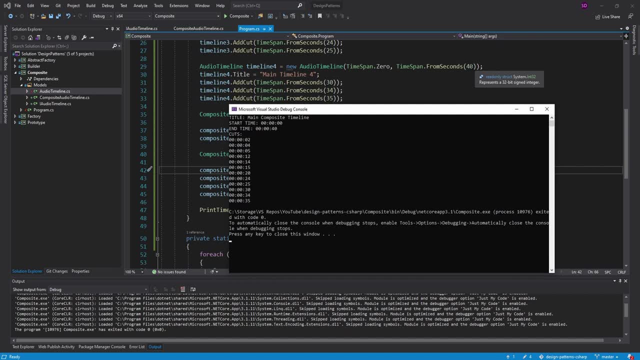 So this will be the main composite timeline. And there we go. We got our singular title. The start time is just timeSpan.0.. The end time is the latest end time from all of my other timelines, So 14.. 40 seconds. 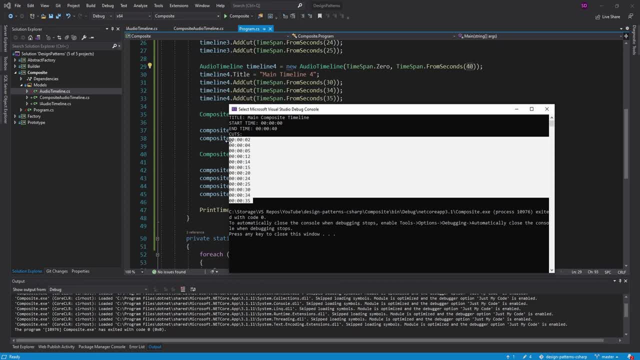 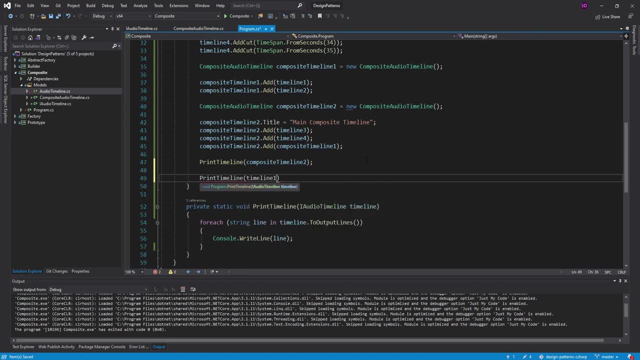 And then we have all of the cuts inside of our timeline And they're ordered as well. So that looks very neat. And of course we can still pass singular timelines into our printTimeline method, So we'll just throw timeline1 in there. 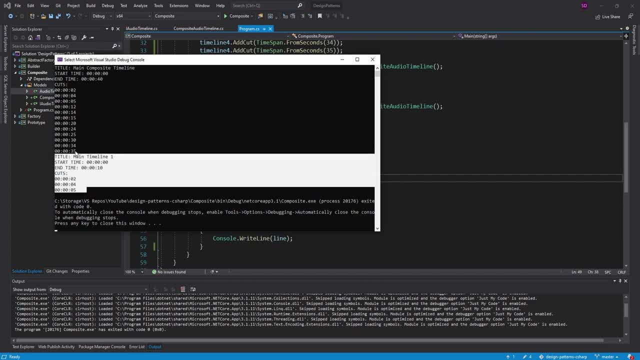 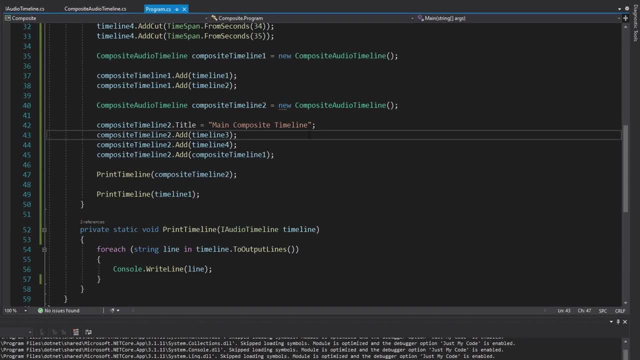 And there we go. We get our single timeline working just as well as our composite timeline. So that is the power of the composite pattern. Our composite group of audio timelines implements the same functionality as our individual audio timeline, So we can simply pass it. 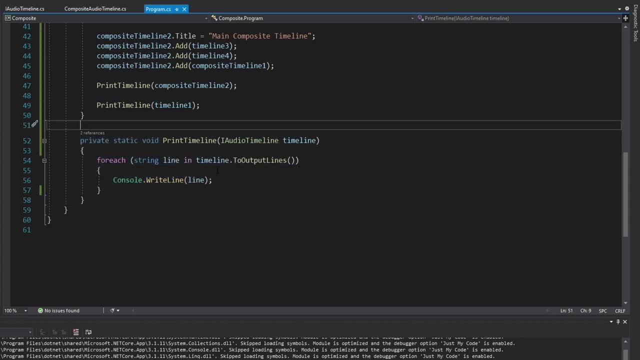 to this printTimeline method, And this method doesn't really care if it's dealing with a composite or an individual audio timeline, And it makes this method much easier to implement. We don't have to do any type checking or iterating over any of the sub-timelines. 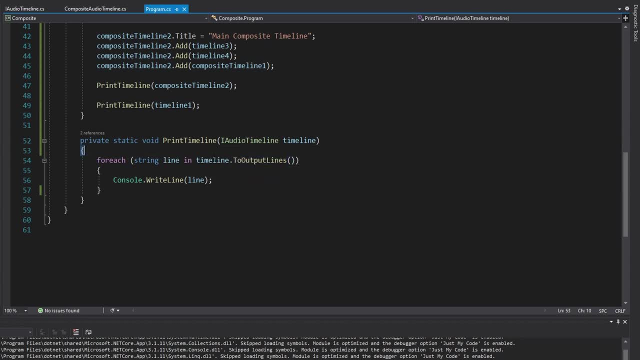 We simply just get the output lines for the timeline. So hopefully you all can use this structural design pattern in your own applications to simplify your clients or services that might want to deal with either a singular or a group of objects. If you have any questions, criticisms or concerns,